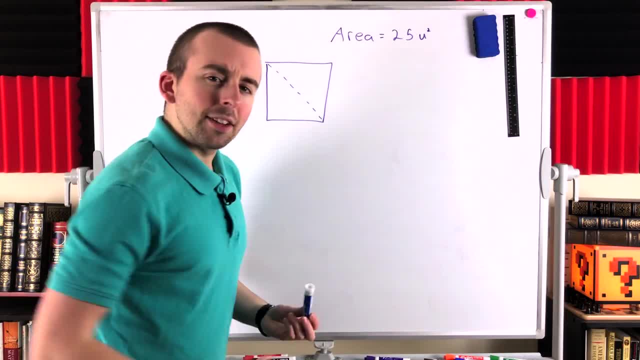 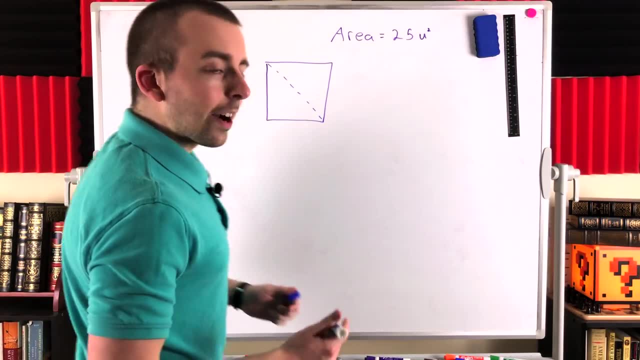 Now, immediately upon drawing the diagonal, just to start visualizing our problem. you should get some hint of how we can solve this problem. Remember that all of the angles in a square are right angles, so, of particular interest, this one here is a right angle. 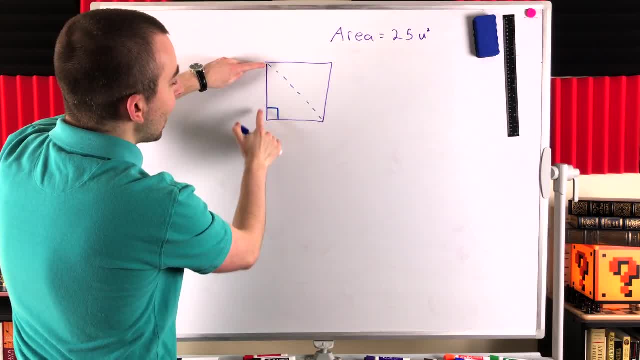 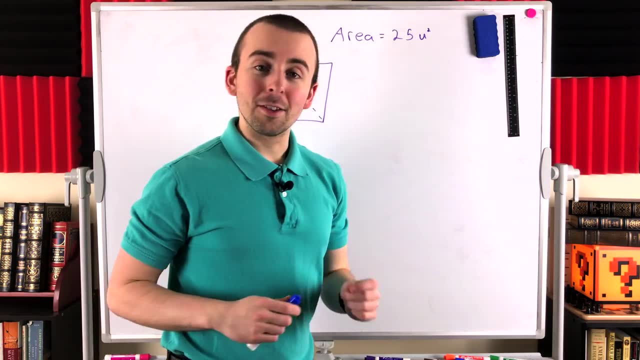 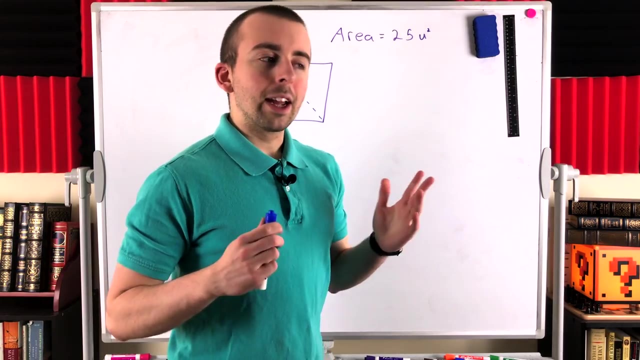 So by drawing this diagonal, we've just defined a right angle. So then, you might think, does Pythagorean theorem, is that going to help us out here? And as it turns out, it will, As it often does. Now, the way your thought process might go to solve this problem is: okay, we've got the area of a square. 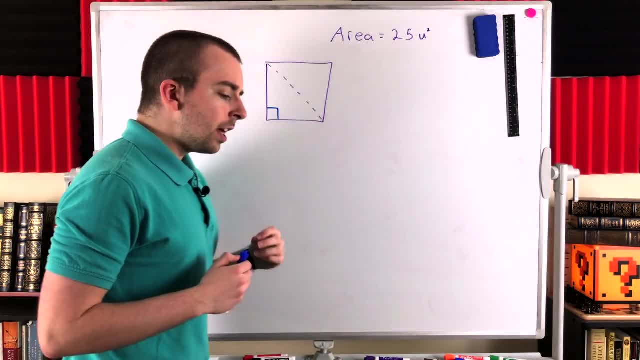 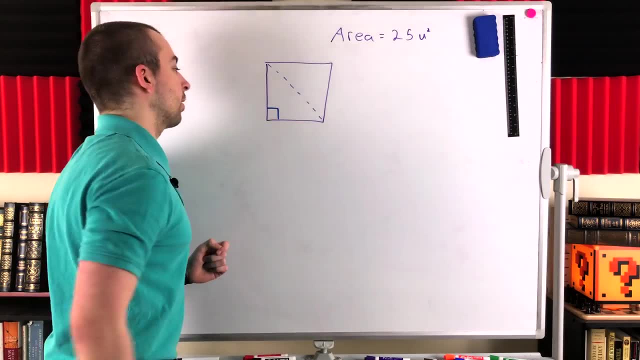 we want to find the length of the diagonal. So do we know? have we solved the similar problem with the same unknown, the unknown being the length of the diagonal of a square? And one that might come to mind is a problem where we're 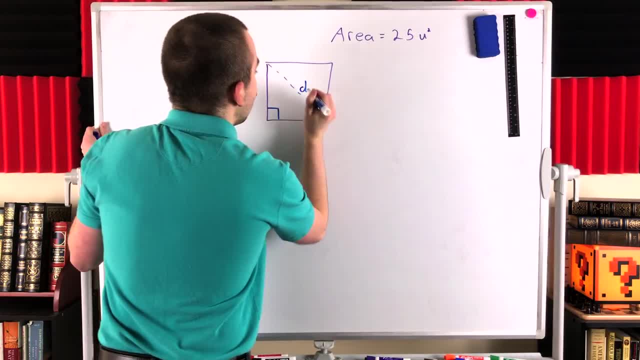 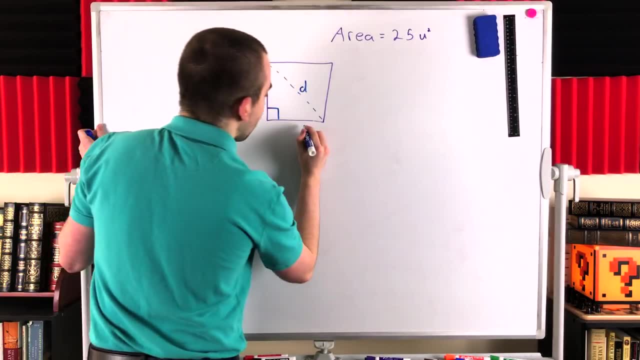 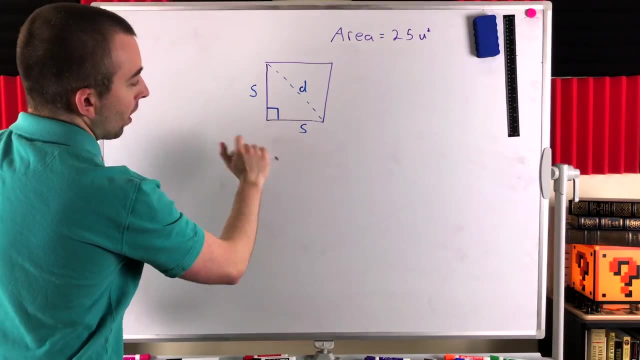 given a side length of the square and we want to find the diagonal from that information. Of course all of the sides of a square have the same length, so if this side is s, this side is also s, and look at that. to find the diagonal from this information we just use the Pythagorean theorem s: squared plus. 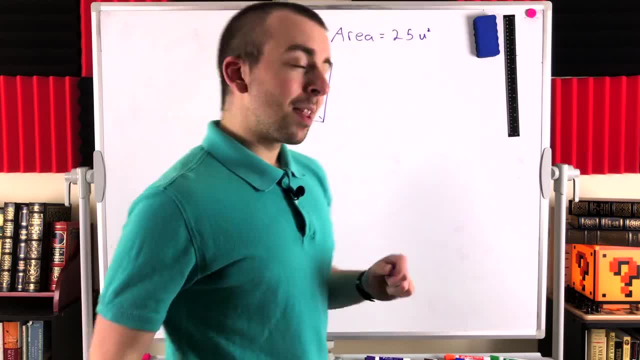 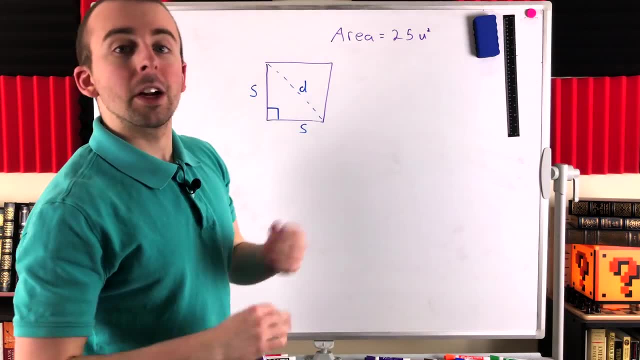 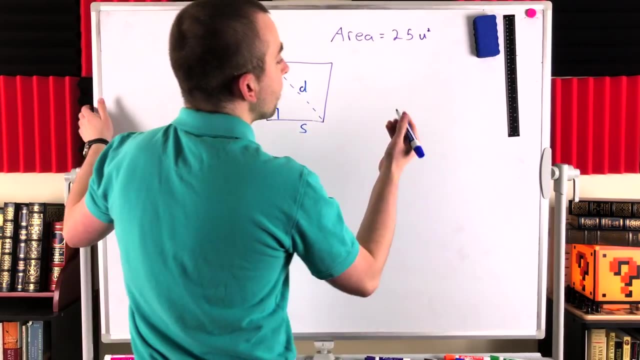 s squared equals v squared. bada bing, bada, boom, there's your answer. So if we can get the side length of the square from the area, then we're back in familiar territory, a problem that we've all probably already done. So can we get the side length from the area? of course we can, because the 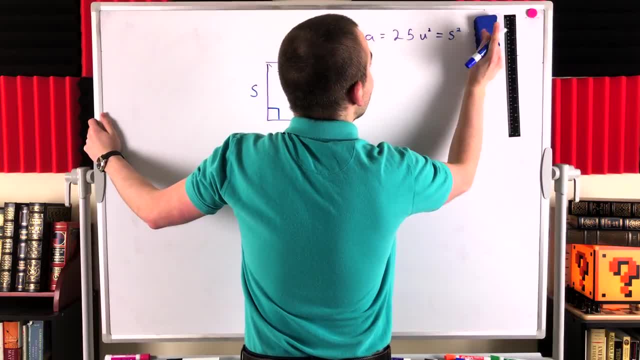 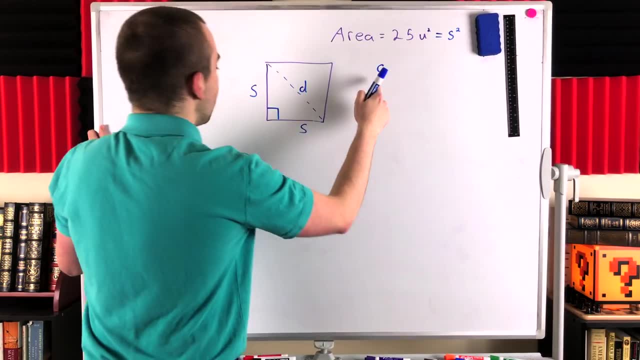 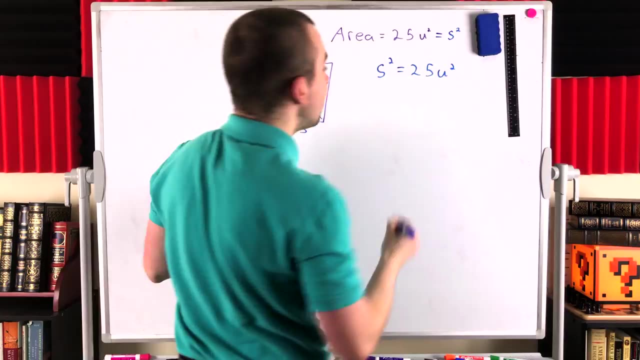 area of a square is just the square of its side length. so if the side length is s, the area is s squared. so in particular we have that. we'll write this: s squared is equal to 25 units squared and just take the square root of both sides and that will give us our side length, and then we can. 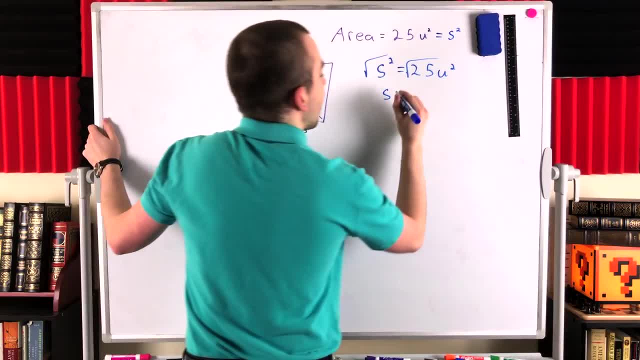 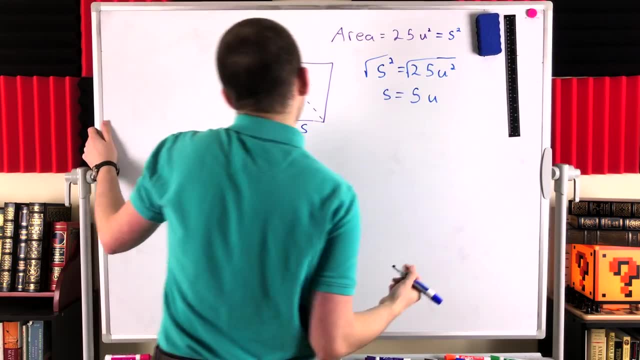 go ahead and use the Pythagorean theorem. so we have that the side length sX over VX squared. and then we can go ahead and use the Pythagorean theorem. So we have that the side length s, s is equal to the square root of 25 units squared, which is just five units. So then we can erase. 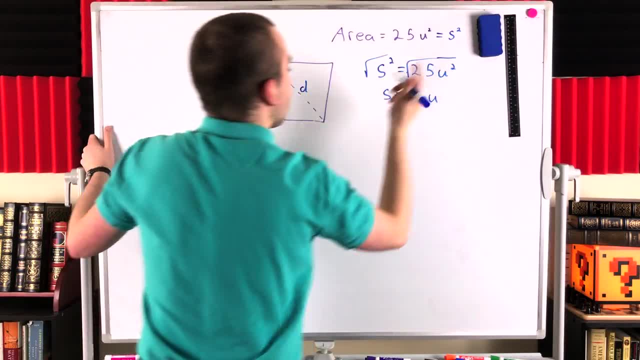 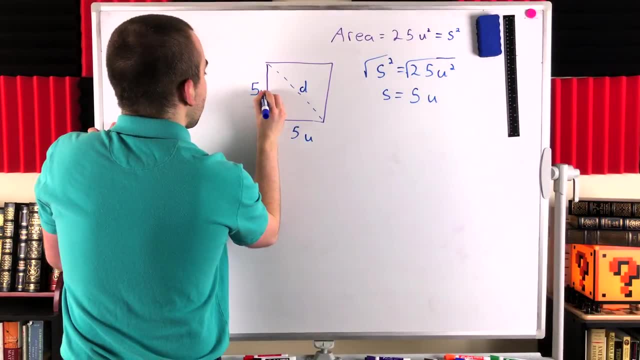 these s's. We know what s is equal to. now, The side lengths of our square five. Remember, all the side lengths are the same, so they're all five. We could go ahead and throw a? u in there, So it's. 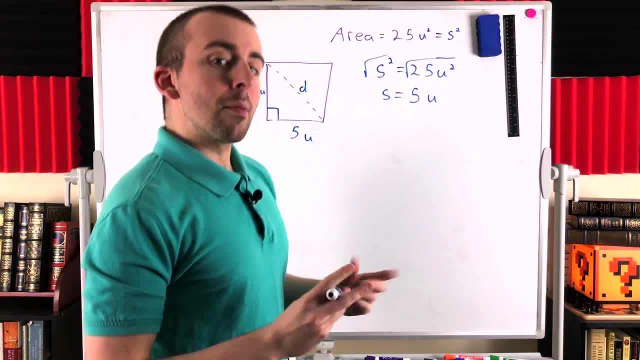 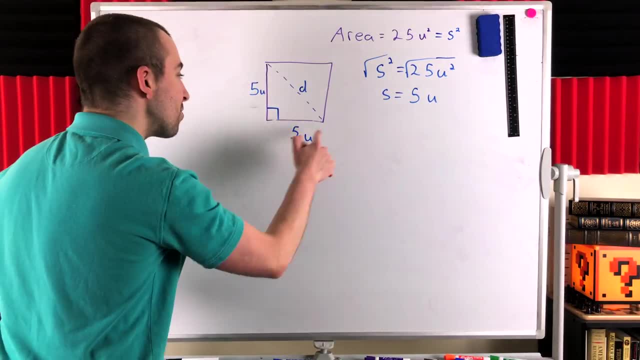 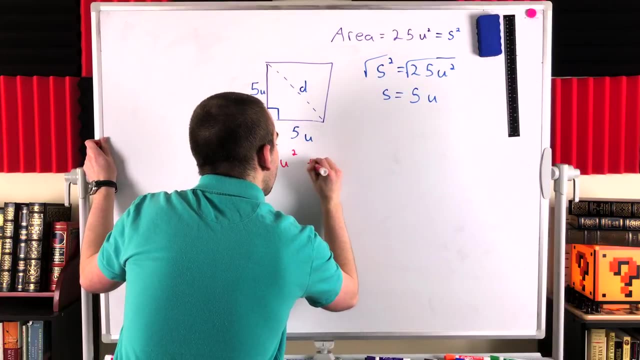 five units, five units. and we just use the Pythagorean theorem, Remember? the Pythagorean theorem tells us that the sum of the squares of the legs of a right triangle is equal to the hypotenuse squared. So we've got that: five units squared plus five units squared. this is all. 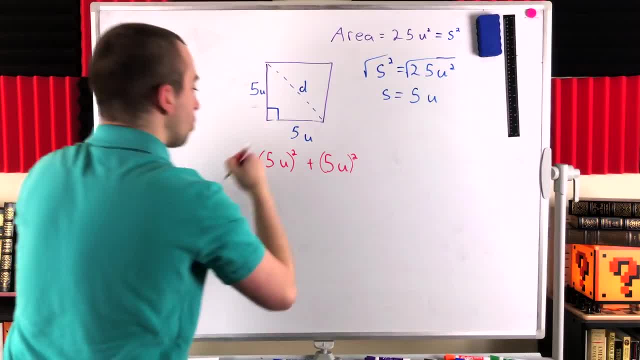 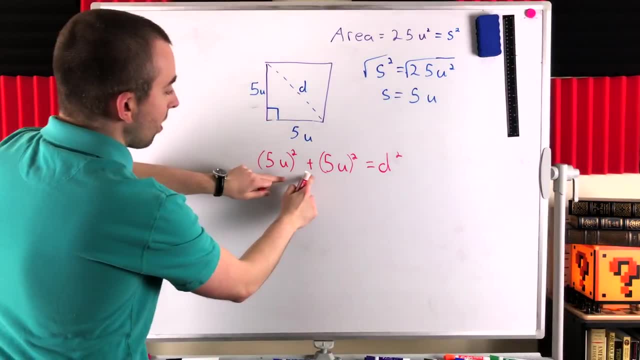 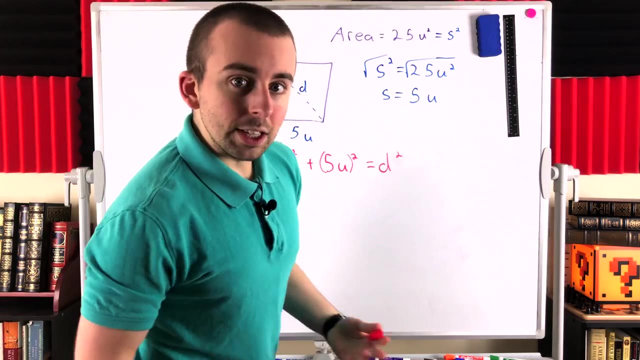 getting squared. five units squared. five units squared is equal to the square of the hypotenuse, which is the diagonal in this case. Again, that's, the sum of the squares of the legs is equal to the square of the hypotenuse. five units squared is 25 units squared. We already 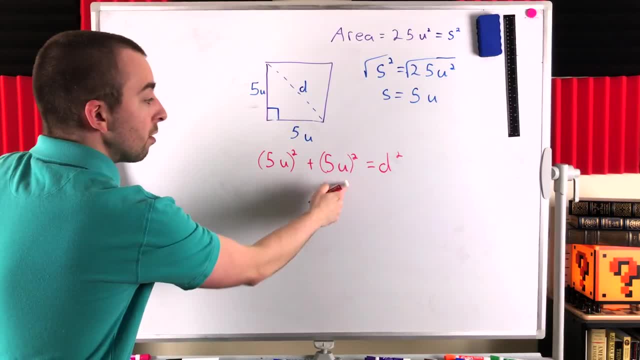 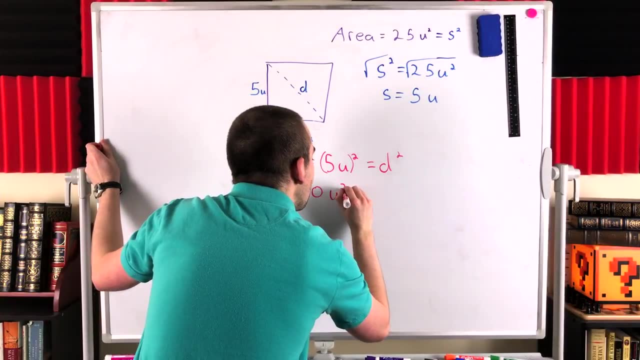 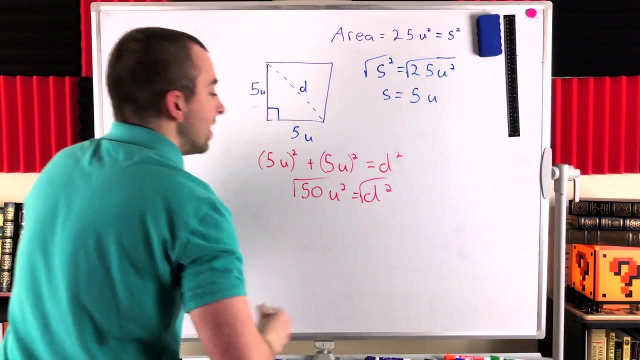 saw that up here. So 25 units squared plus 25 units squared, that's 50 units squared, And so we're almost done. We've got that 50 units squared is equal to d squared. Just take the square root of both sides here, and we've got that the diagonal d is equal to the square root of 50 units. 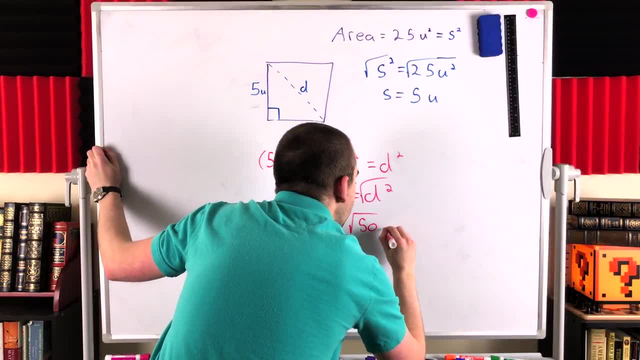 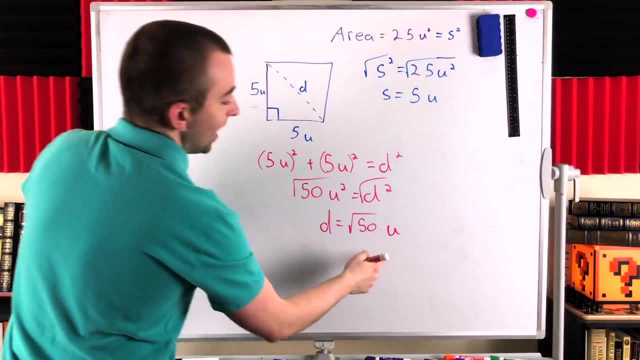 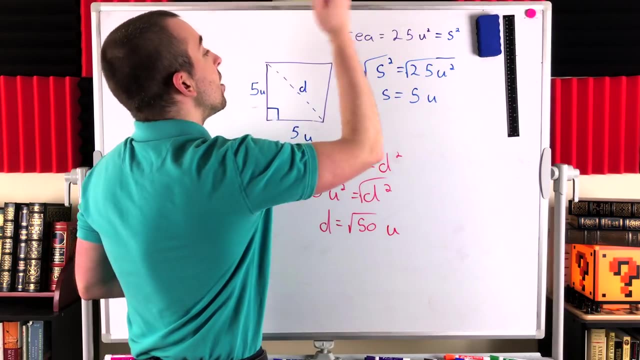 squared, So we could just write that as the square root of 50.. And then the square root of units squared is units. So this is just the square root of 50 units And that units is outside of the square root, And that is an exact answer. So if the area was 25 inches squared, then 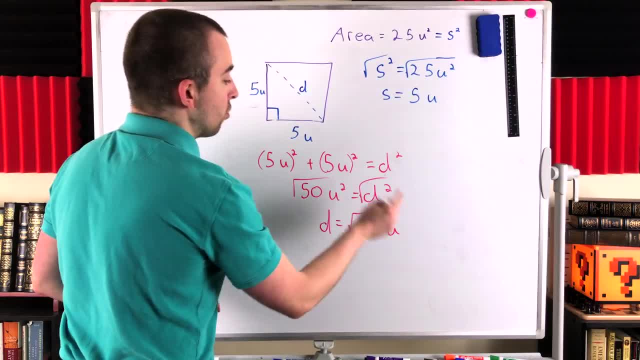 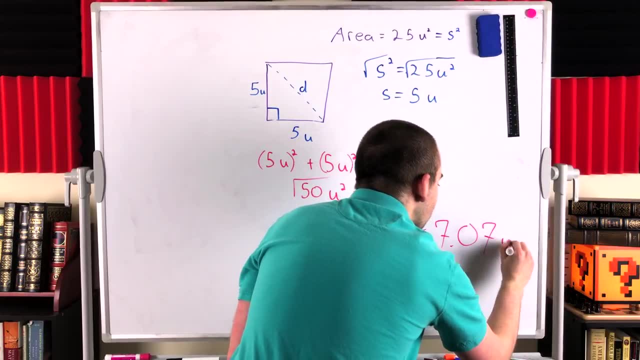 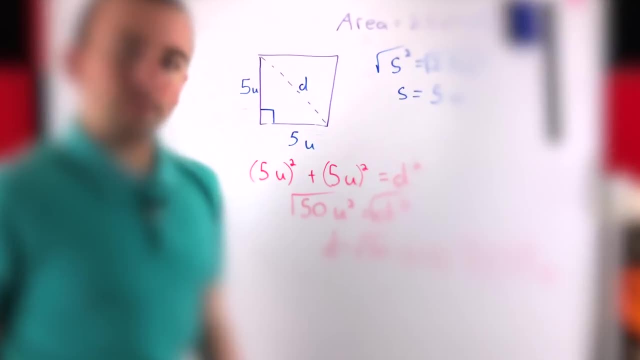 the diagonal is root 50 inches And we could approximate this if we wanted to. It's about 7.07.. Just pausing here for a moment to point out that this same exact procedure would give us the same exact result if we were trying to find the other diagonal of the square. 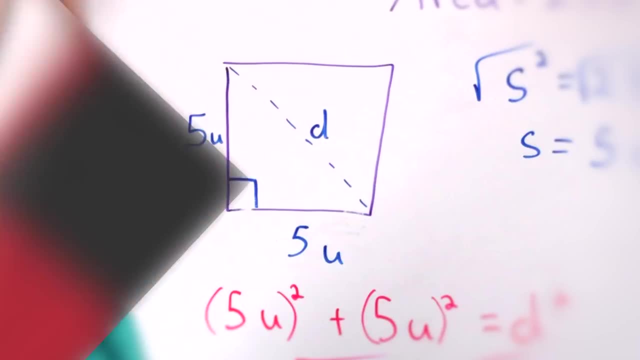 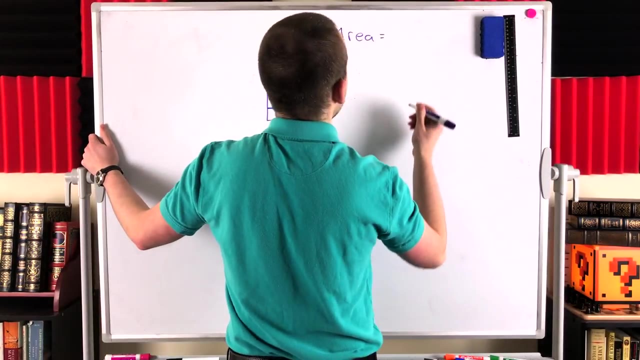 the one that goes the other way. All right onto the rest of the lesson. So I want you to try this one on your own before watching the solution. Let's say we're given that the area of the square is 16.. We'll say we'll work with an actual unit this time. So say: 16 centimeters squared. So go ahead and write that down And then we'll try to find the area of the square. Let's say we're given that the area of the square is 16. And we'll say we'll work with an actual unit this time. So say, 16 centimeters squared. So go ahead and 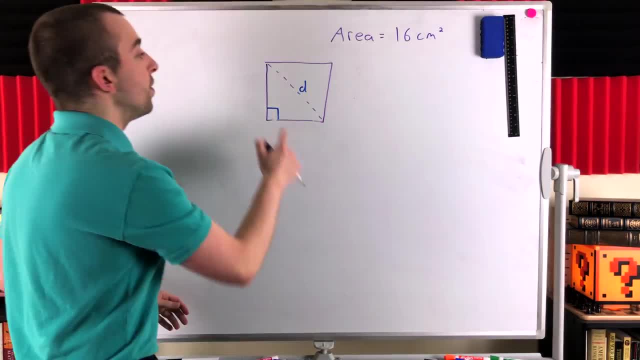 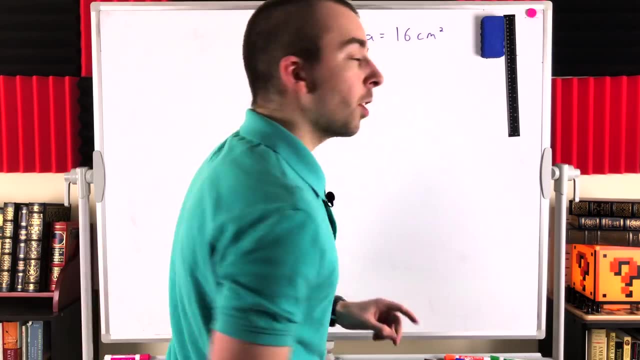 solve this problem, just like we did before, to find the diagonal of a square that has an area of 16 centimeters squared. All right, hopefully you've got an answer Now when I go through this problem. I'm going to leave out the units Once you do a couple of these. 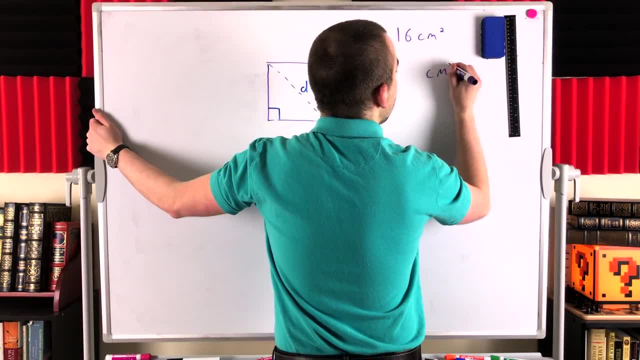 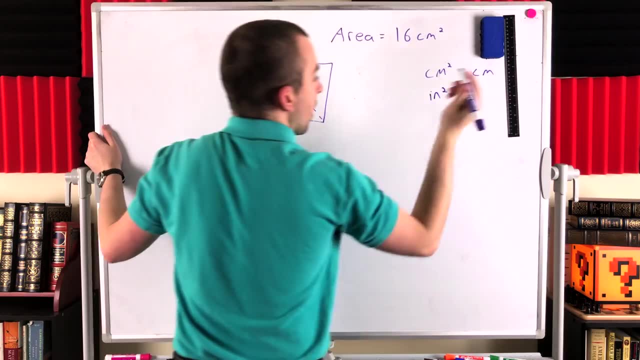 problems. you know that if you're given an area in centimeters squared, for example, your side length is going to be in centimeters. If you're given your area in inches squared, your side length is going to be in inches, and so on. 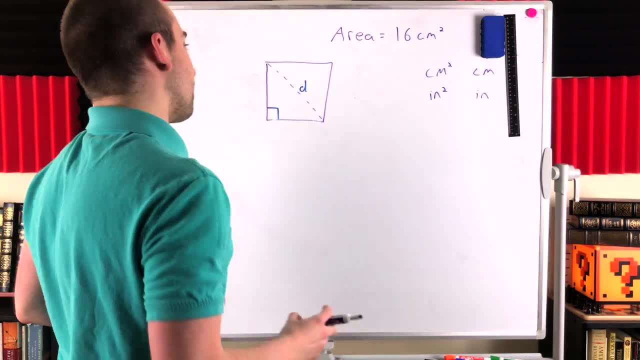 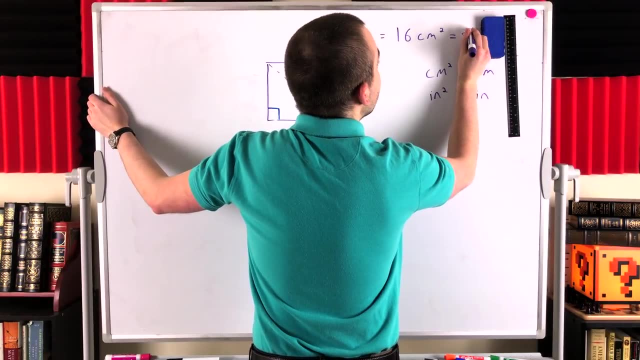 So we can leave off the units. We know what the units will be at the end. So how do we solve this problem? Same way we did before. The area is 16 centimeters squared, which is the square of the side length of the square. So then we just take the square root of both. 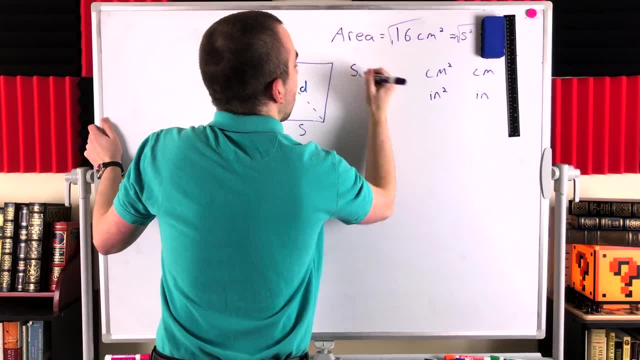 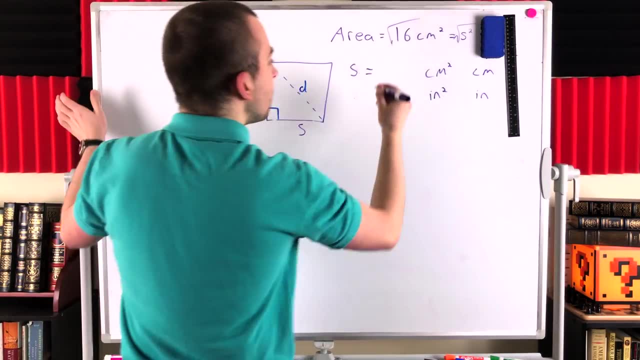 sides Square root of that, Square root of that. So, leaving off our units, we have that the side length of the square is equal to the square root of 16.. What's the square root of 16?? Well, of course that's 4.. So then we can go ahead and erase that square root. 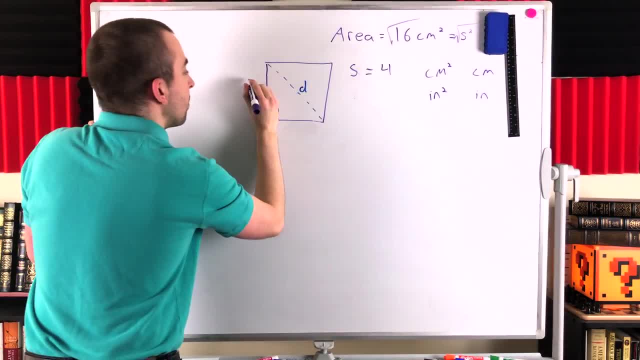 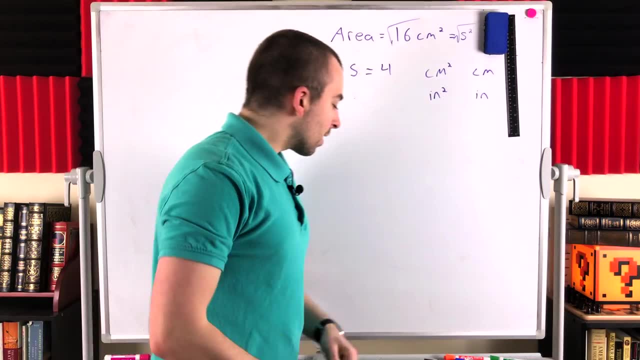 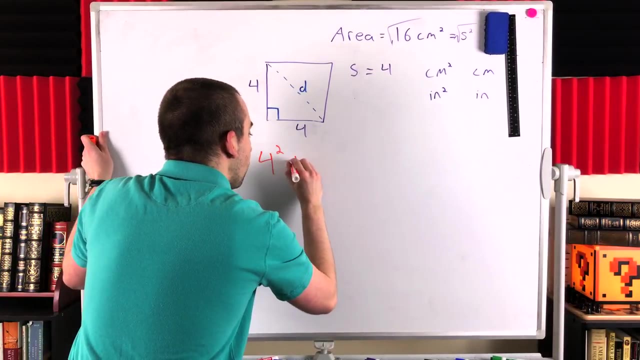 Erase our s's over here. We know that the side lengths of this square are all 4.. Now we've got a right triangle with leg lengths of 4.. We just go ahead and apply our favorite Pythagorean theorem that tells us that the sum of the squares of the leg lengths 4 squared. 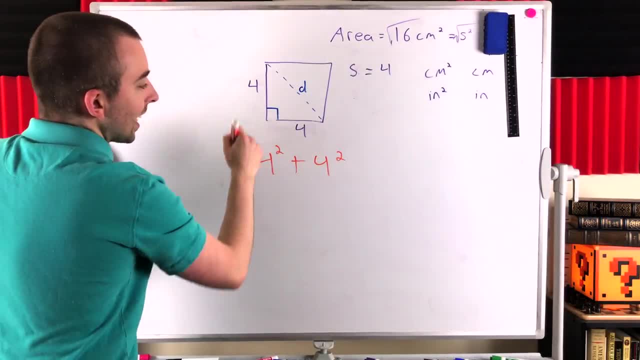 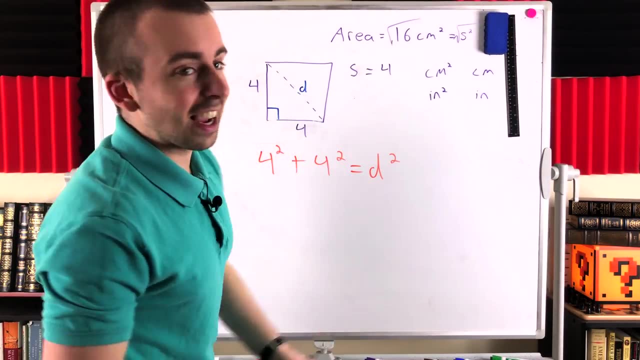 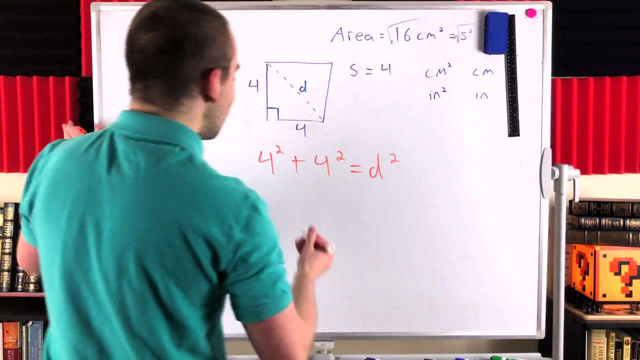 plus 4 squared, that's the sum of the squares of the leg lengths, is equal to the diagonal squared d squared, or the hypotenuse, which in this case is our diagonal, That we're looking for. 4 squared plus 4 squared, that's 16 plus 16, and that is 32.. So 4. 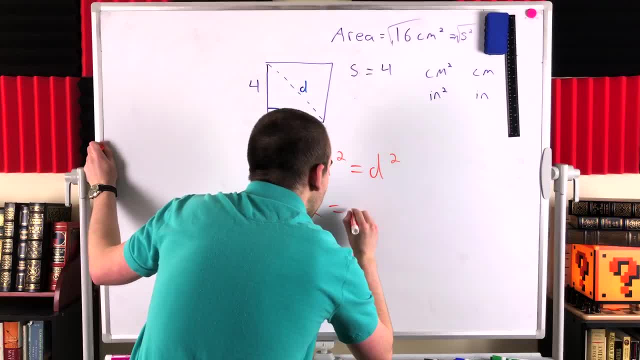 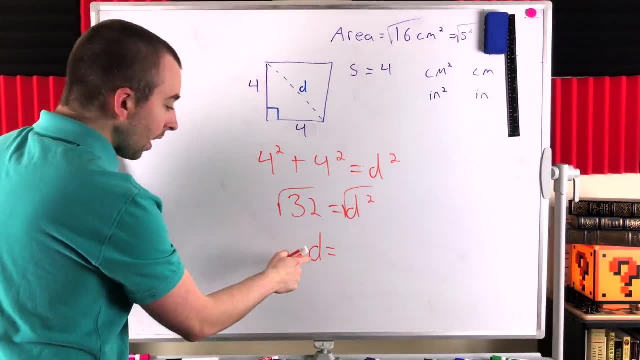 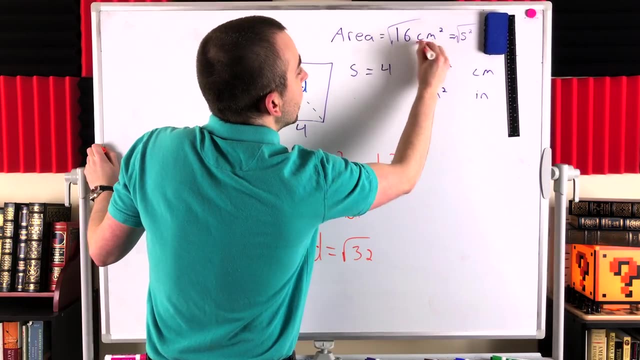 squared plus 4, squared 16 plus 16,, that's 32, is equal to the diagonal squared. Take the square root of both sides and we've got our answer: The length of the diagonal of the square is equal to the square root of 32.. So, since our area was given in centimeters, 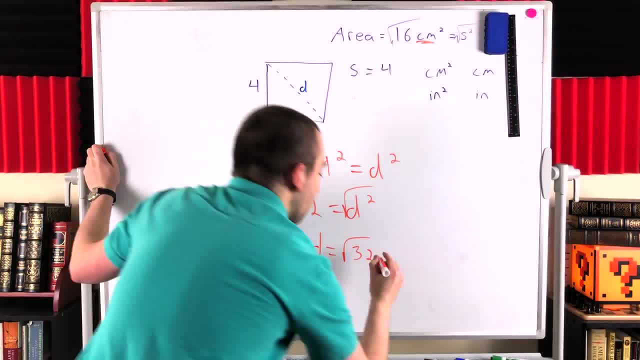